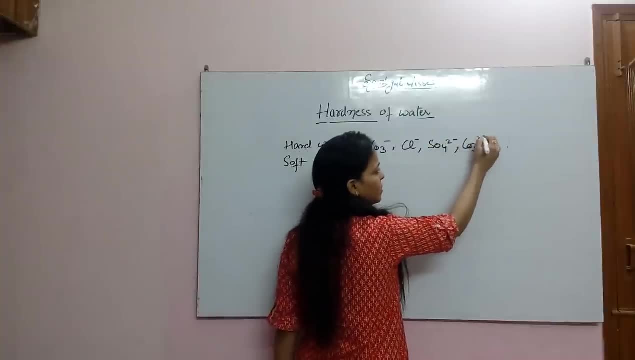 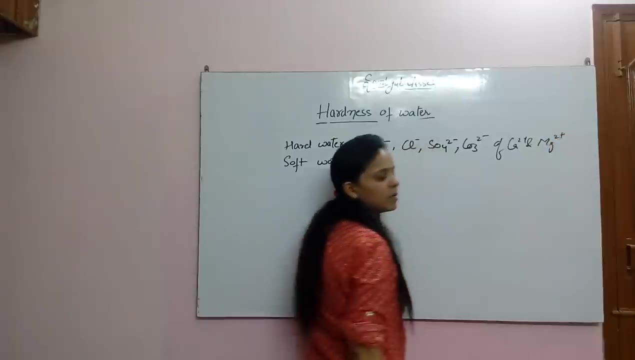 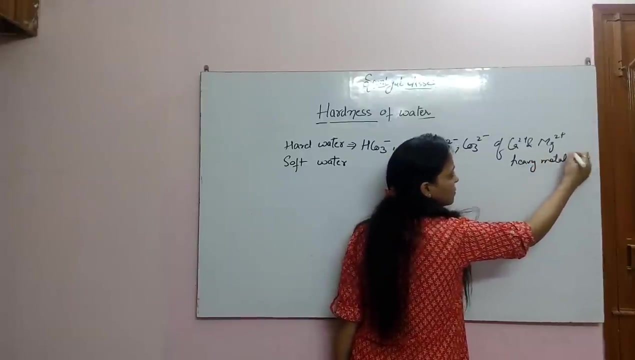 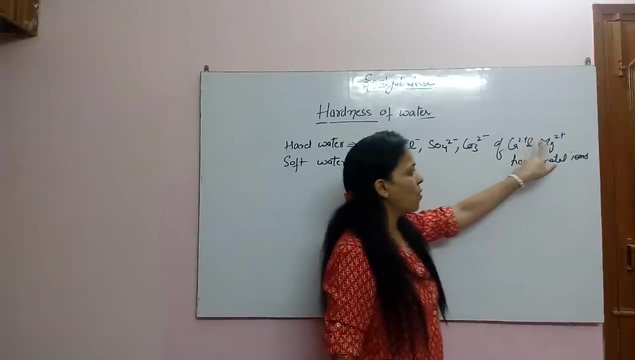 ions and carbonate ions of calcium and magnesium metal ions, or we can say heavy metal ions. Heavy metal ions. Clear Hard water means a water in which calcium and magnesium metal ions are present. Which ions are present in it? Calcium and magnesium metal ions are present. 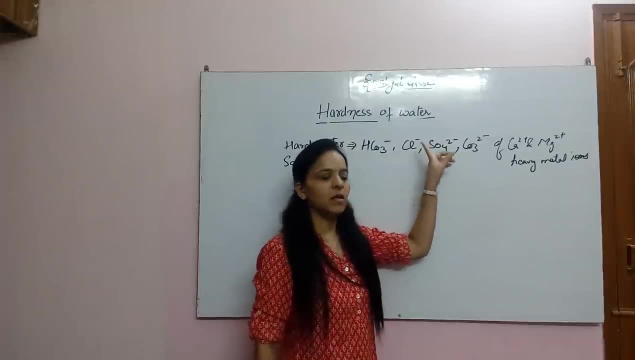 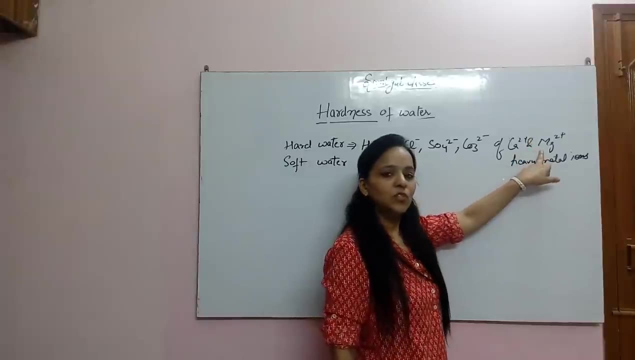 So why are the ions present in it? Because there is a water in which a bicarbonate chloride, sulphate and carbonate ions are present, A water in which calcium magnesium and metal ions are present. What are the ions present in any heavy metal? ions, bicarbonate chloride. 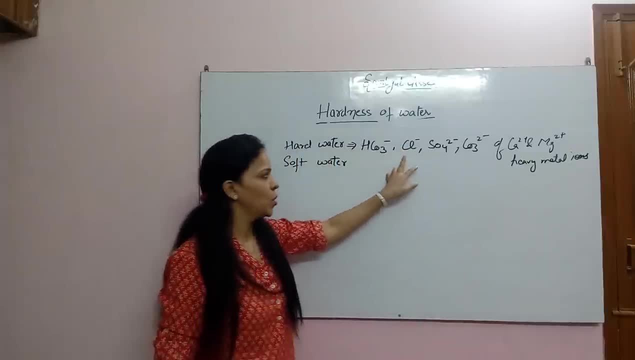 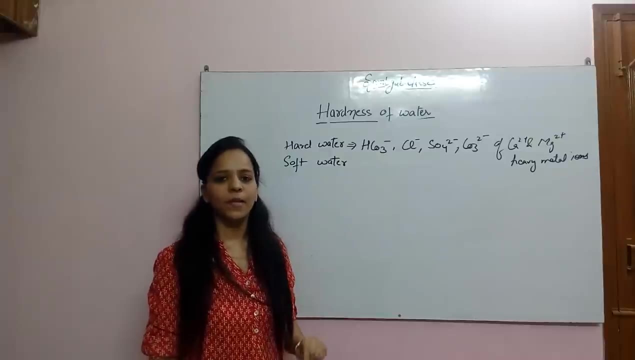 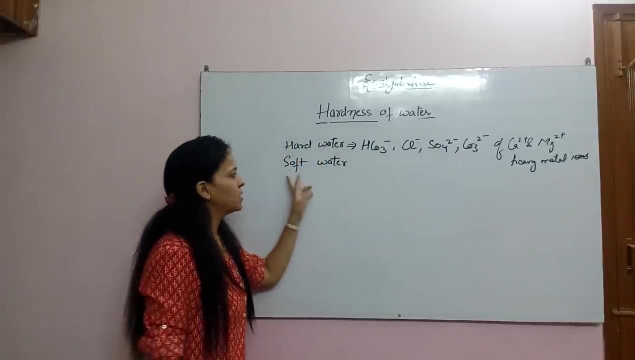 sulphate and carbonate, ions are present. So it means that water is hard water, The water which is free from all these ions, A water in which so many things are present and hence All these are free from ions. What kind of water is that? Soft water? 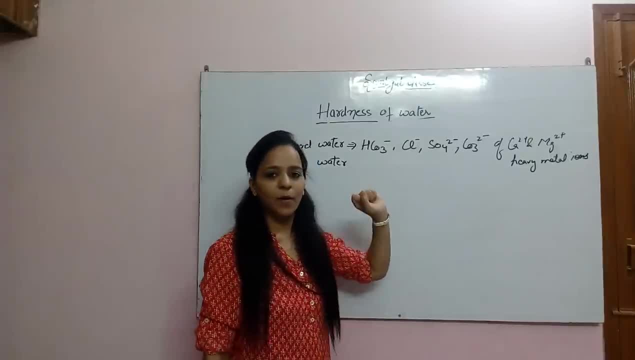 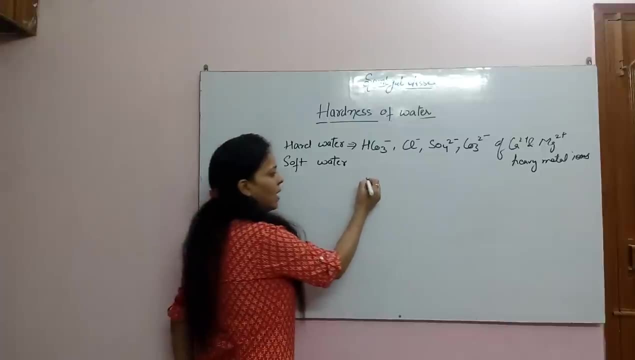 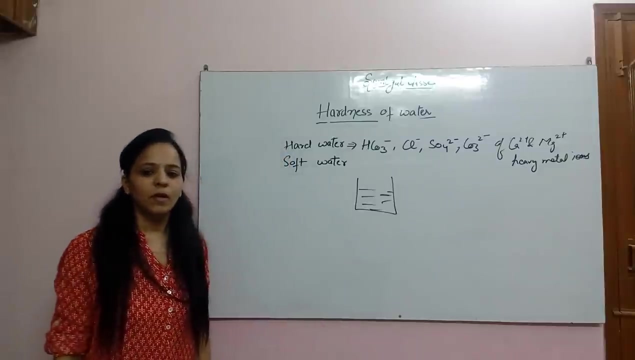 You must have seen it at home. It is called as Khara water. So what we call as Khara water is Hard water. Is it clear, For example, if you have Water, What we have put in this Water? Now, what is in water? 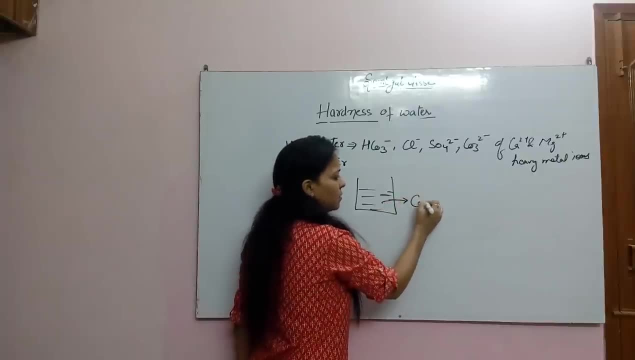 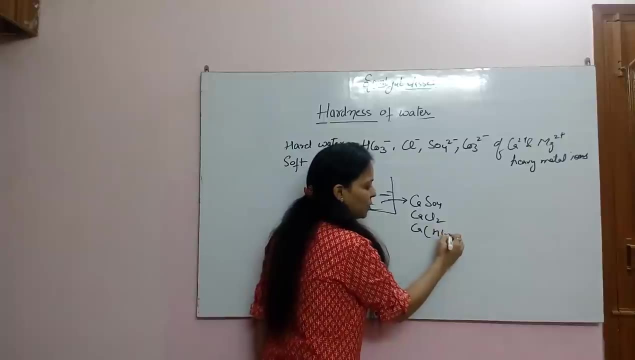 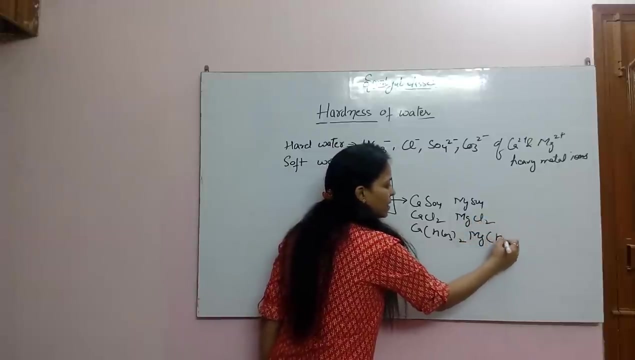 If in this water Calcium Sulfate is present, Calcium Chloride is present, Calcium Bicarbonate Is present, Magnesium Sulfate is present, Magnesium Chloride is present Or Magnesium Bicarbonate is present, Then this water is known as. 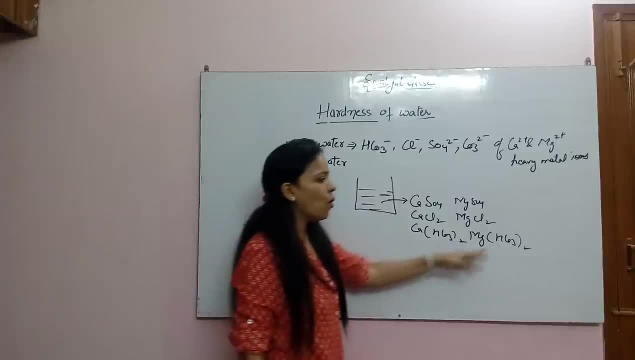 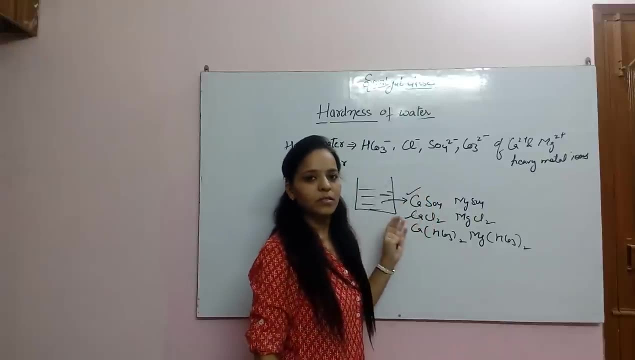 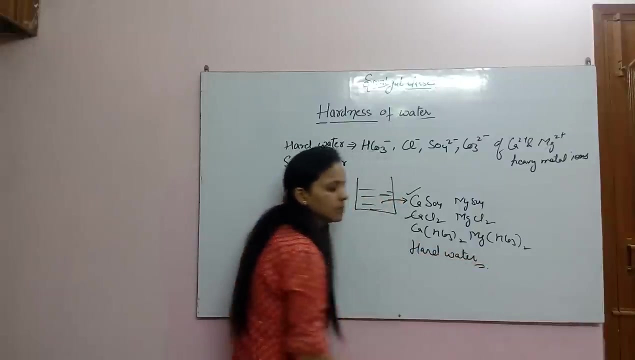 Hard water, Water which contains all these Salts. It is not necessary that all the salts From these One salt, two salts or all the salts Which is present in the water. How will that water be Hard water? Is it clear? 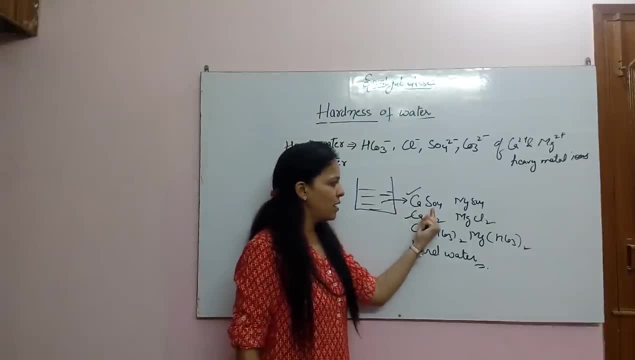 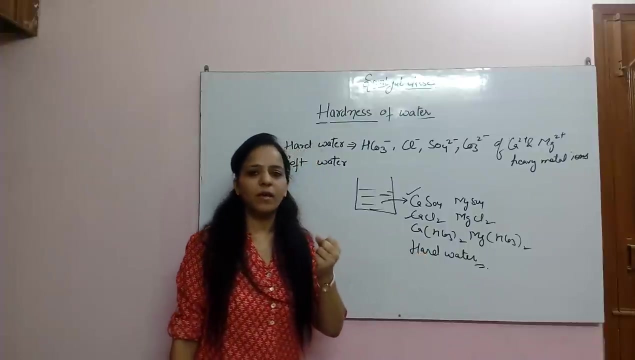 Means Such water in which Calcium and Magnesium Is present: Sulfate, Chloride, Bicarbonate Or Carbonate. Such water we will call Hard water, Which we call at home Khara water. Why is Khara water? Because these salts are present in it. 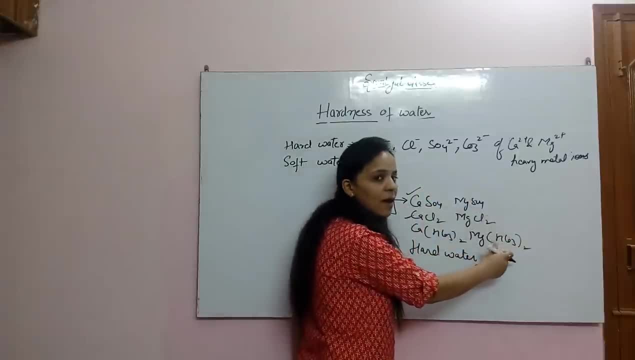 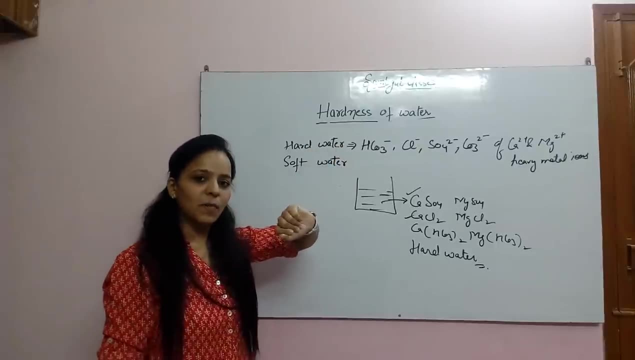 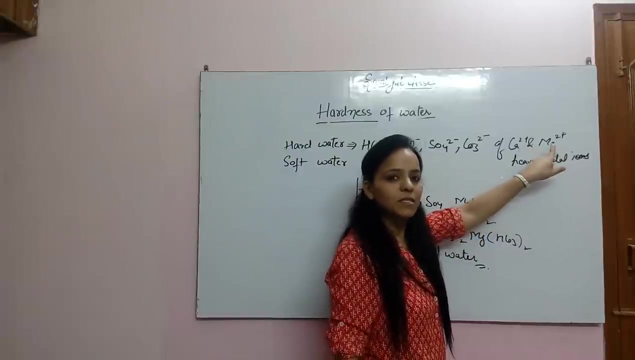 All these salts are Responsible for Hardness. Now we will see Hardness. Soft water Is known. Hard water is Such water in which Bicarbonate, Chloride, Sulfate And Carbonate are present, Whose Calcium and Magnesium ions are present. 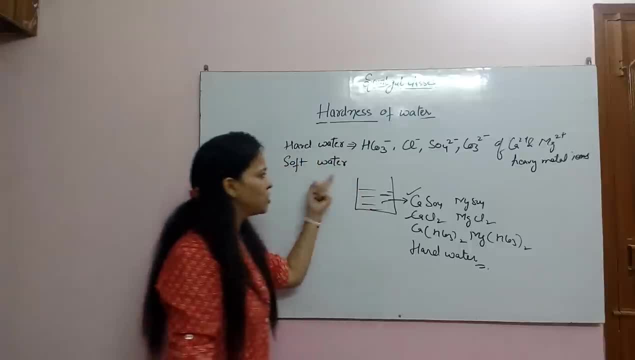 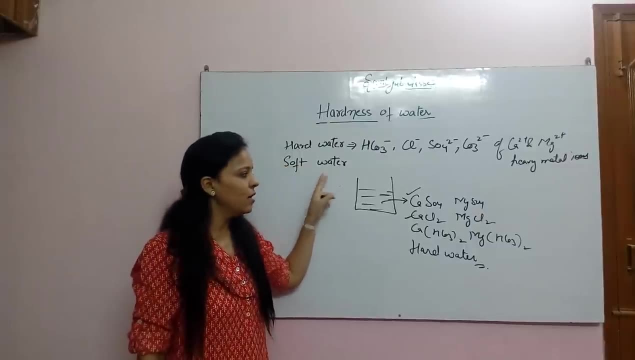 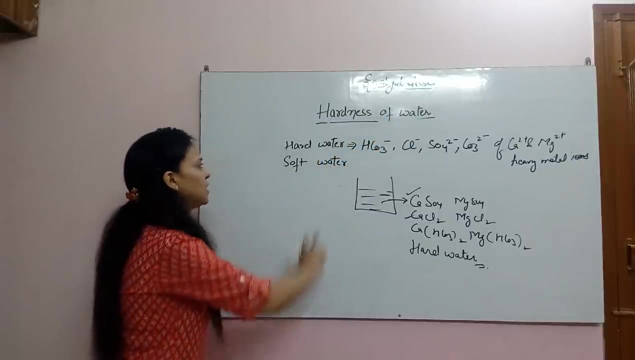 Or any heavy metal ions. And what is soft water? Such water which is Free from all these ions, That is known as soft water. Now see What is hardness of water. First of all, We have read about Hard water, So this property of water, 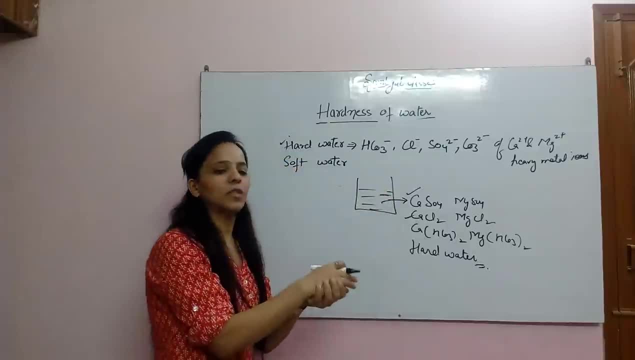 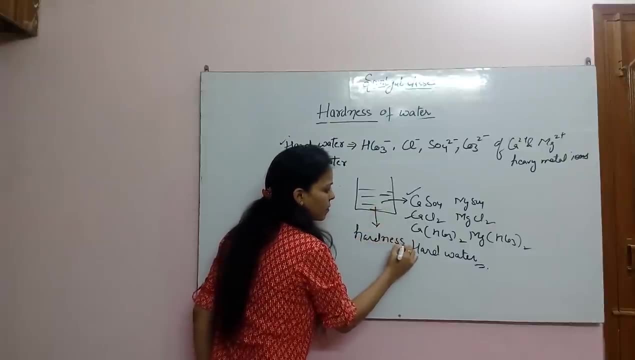 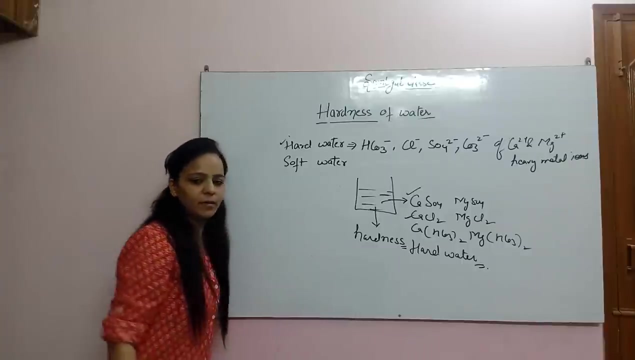 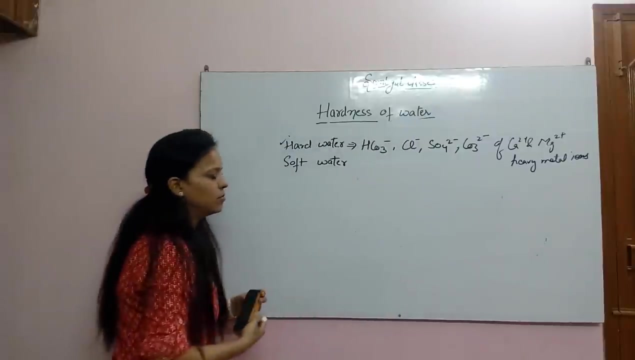 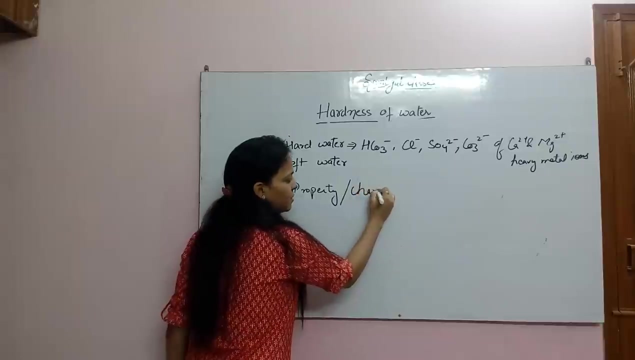 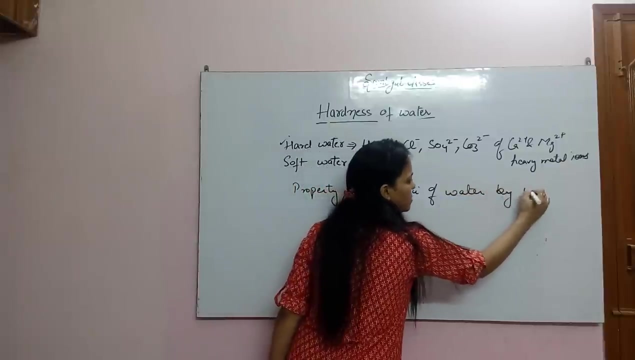 Or we can say: When water is hard, When water is hard, That property we call Hardness. Is it clear? What do you mean by hardness? Hardness means Property. Let's discuss it. Property Or Characteristic Of water. By which, By which, By which? 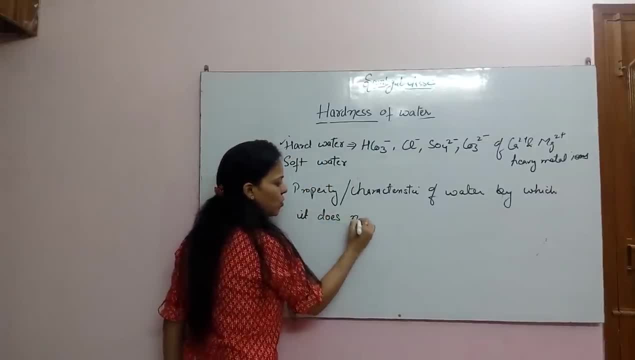 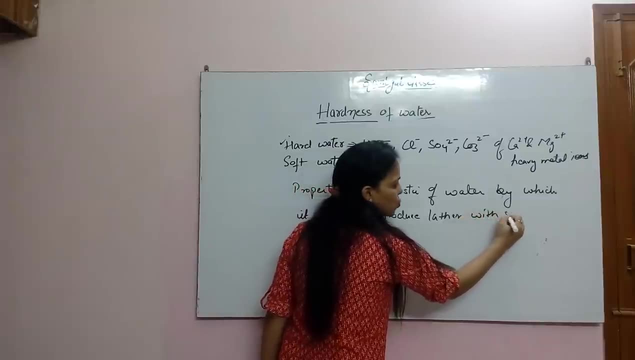 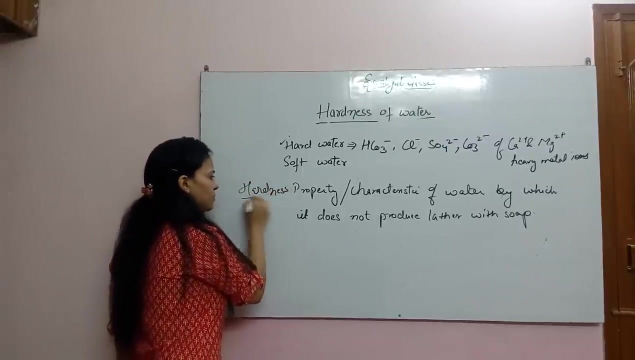 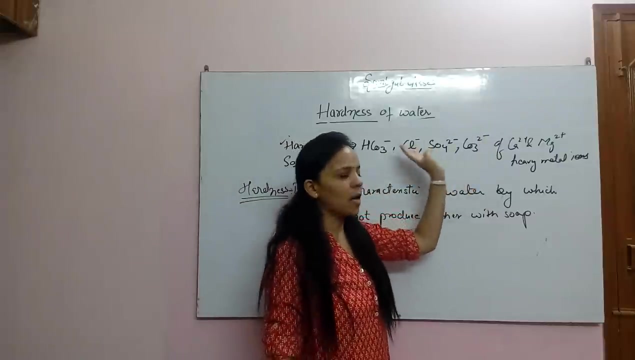 It does not Produce, Does not produce Lethal With. So This is hardness. Let's see once What is hard water: Presence of Calcium Carbonate, Sulfate, Chloride, Bicarbonate Ions in water. That water is known as hard water. 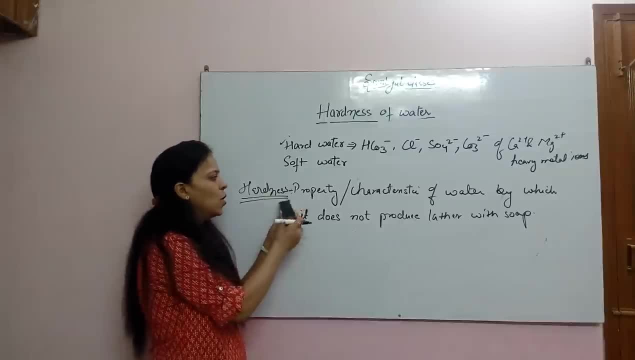 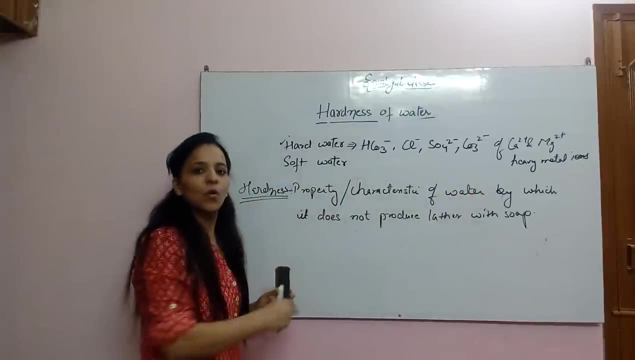 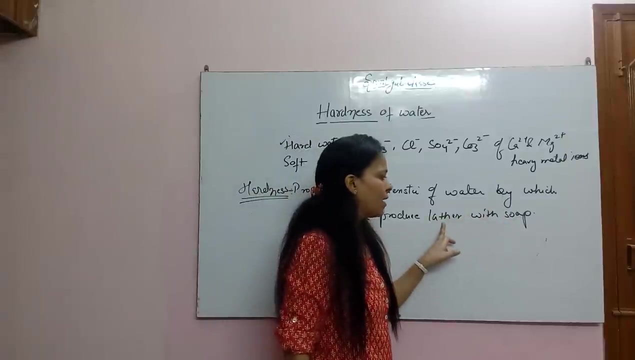 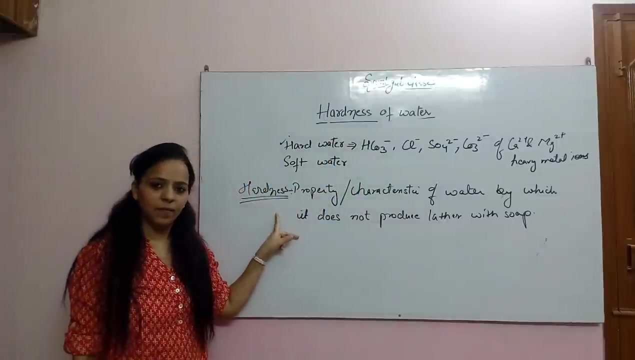 Now, what is hardness? Hardness is the Property of water, Clear Property of water, By which Water that will not produce Lethal with So It means The property of water In which The soap Lethal means foam. The soap does not Produce foam with water. 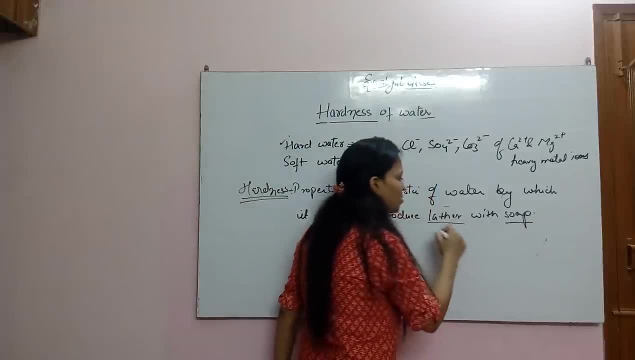 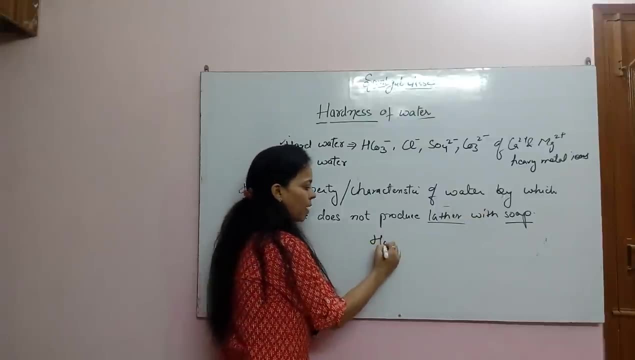 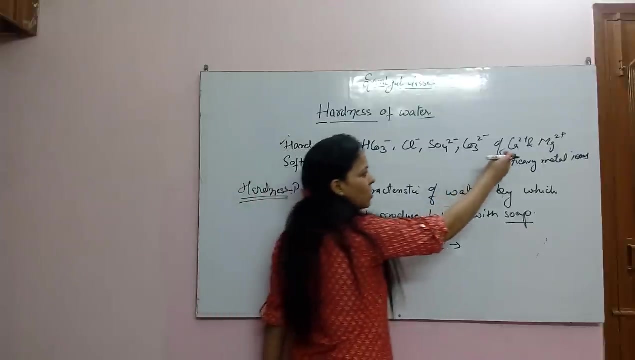 This property we call Hardness Lethal with soap. Why it will not produce foam, Because hard water will be Our hard water. What is present in hard water? All salts are present. So what will these salts do? Combine with your soap And Start making a separate 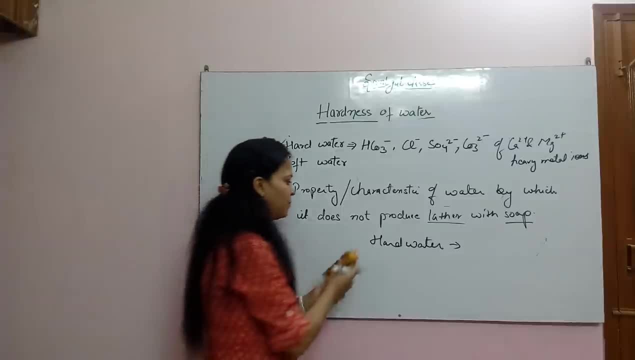 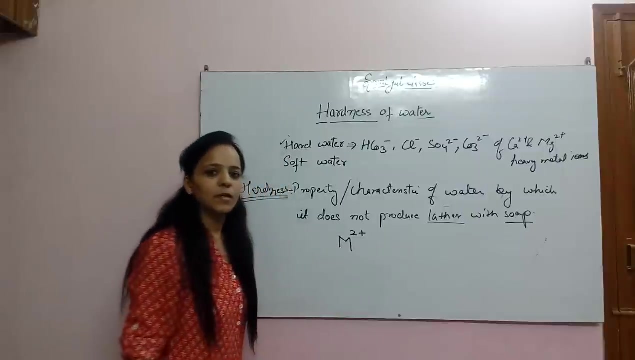 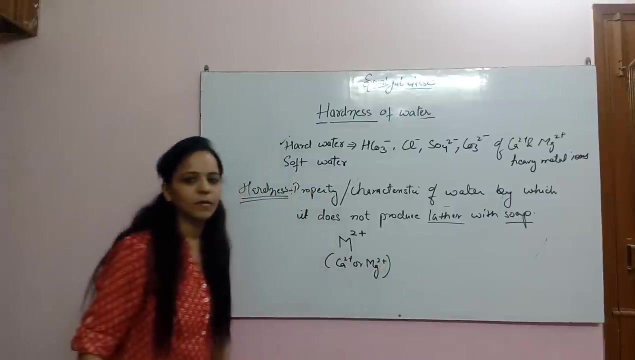 Precipitate. See, for example, What we did at home. For example, We gave water. Suppose our water is hard water. So what will happen in hard water? Any hardness metal Is present, Suppose it may be Calcium iron or Magnesium iron, Clear Metal iron, Any hardness iron. 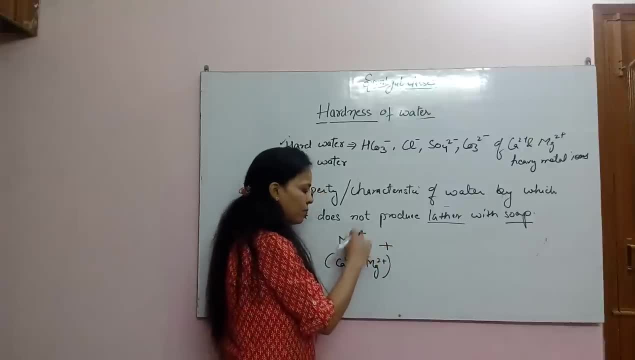 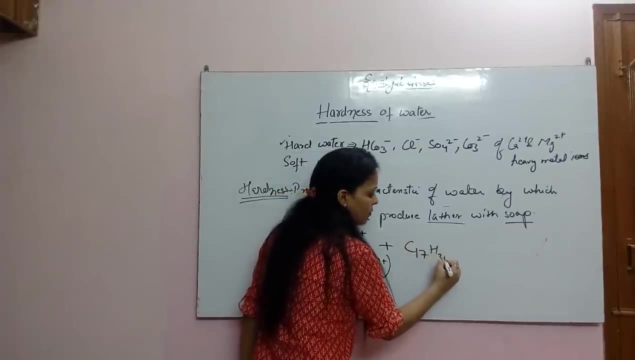 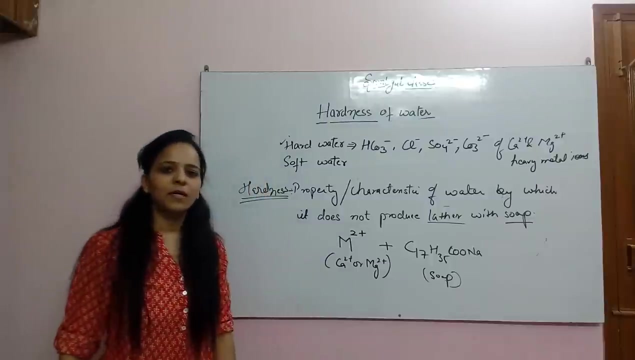 Calcium and magnesium, iron Plus water. We will take water to wash clothes. Now what we will apply? Soap? we take the form of soap C17, H35, COONN, Sodium stearate. This is sodium stearate. Clear, Now what will happen. We are applying soap. 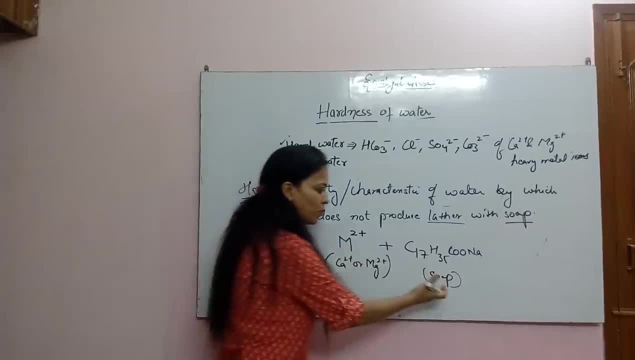 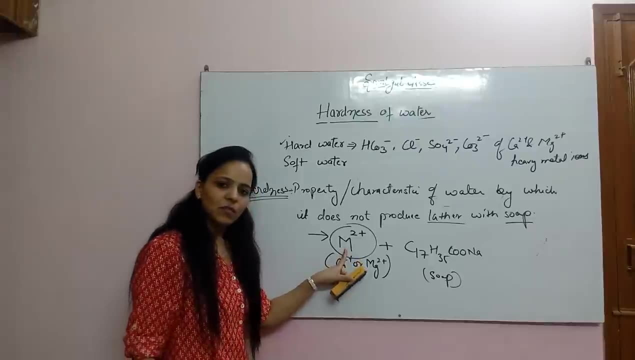 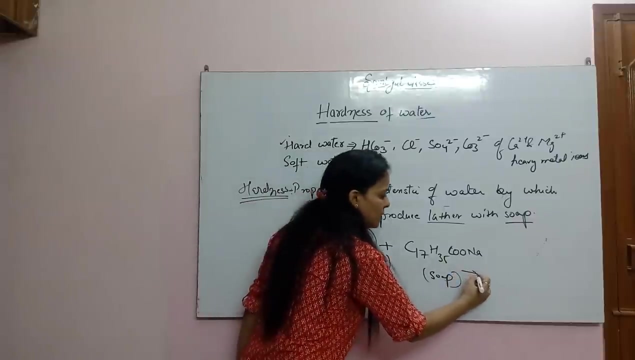 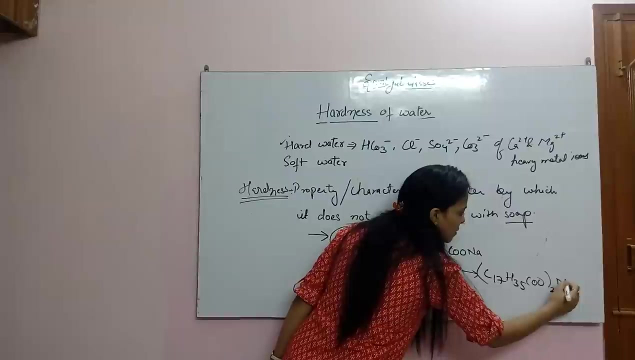 Our water is hard. Now what will happen? Soap that will combine with This metal iron. With this metal iron It will combine To form a sticky Precipitate How- C17, H35, COO- From where metal iron will come. Sodium will be replaced By this metal. 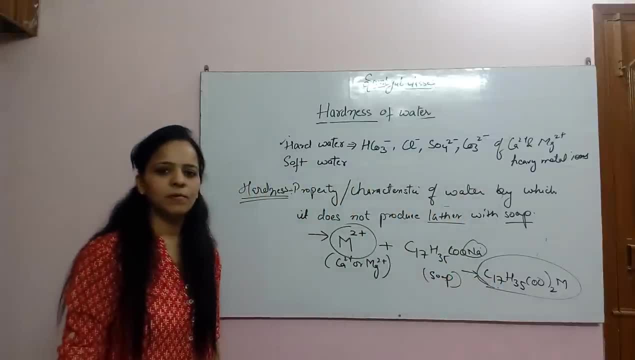 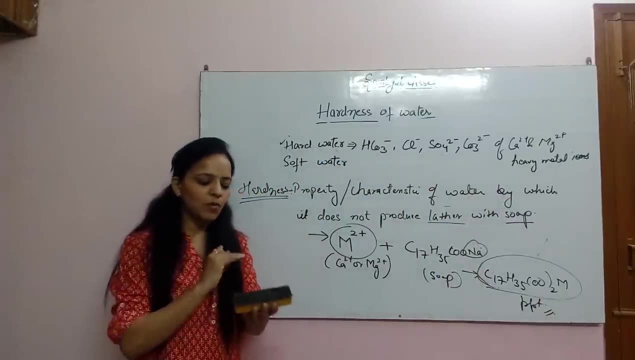 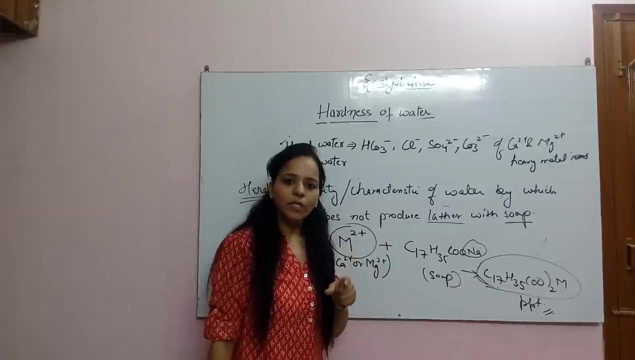 So this will be our resulting Will: be Okay, And these will be PPCs. We say That keep on keeping soap. It is not coming out of the clothes. Why it happens? Because our water is hard water. What will happen in hard water? All these metal irons? 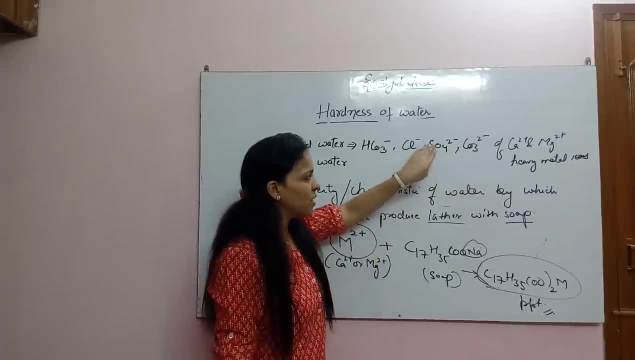 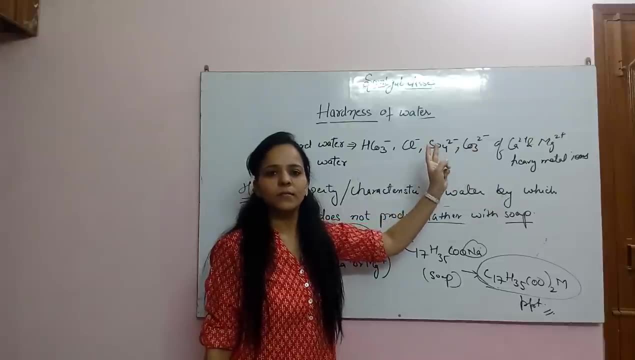 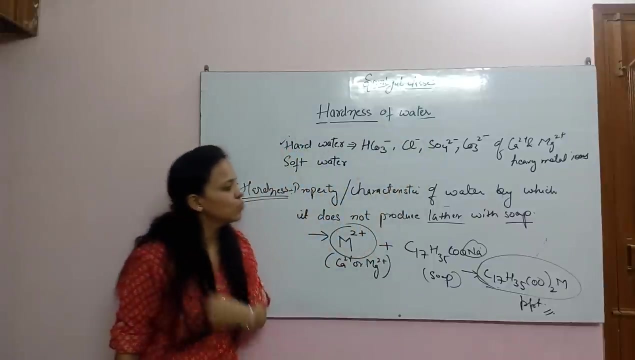 And all these salts will be Because of which hardness is there Now till this is present in water. So what will happen? Soap will keep on combining with them When these metal irons Will be finished, Or the salts- Hardness producing salts- When they will be finished. 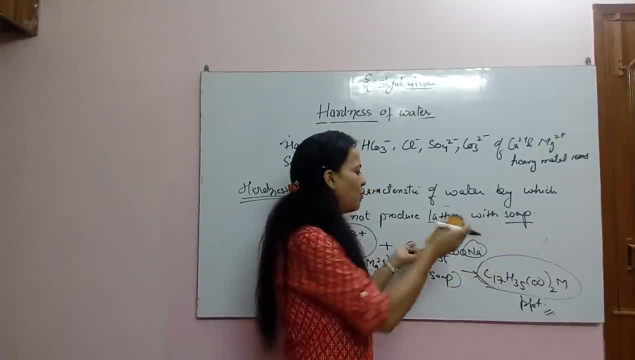 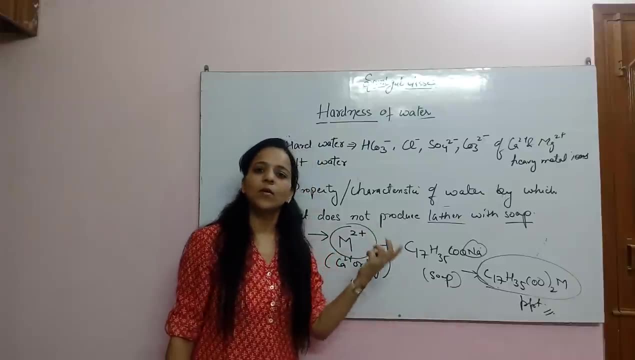 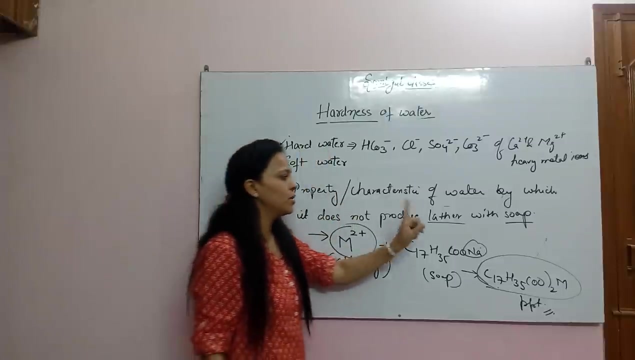 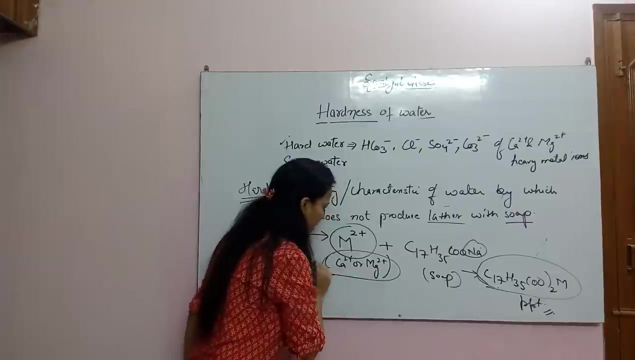 After that, only your soap Will produce leather suddenly. Why? When hardness, metal irons Will be finished, Soap will produce leather suddenly. So that is why The hard water That does not produce Leather with soap. Why Due to the presence of Hardness causing metal irons. 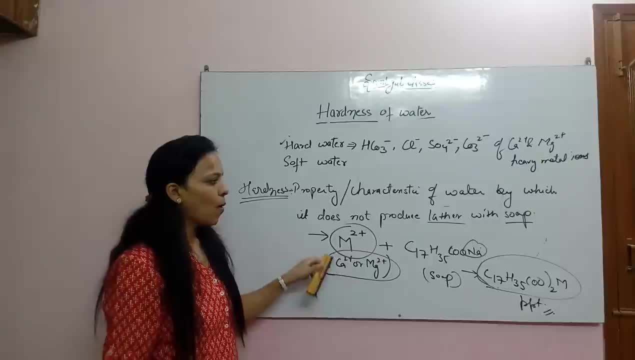 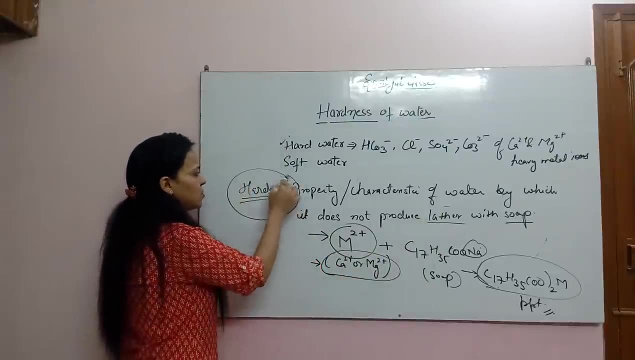 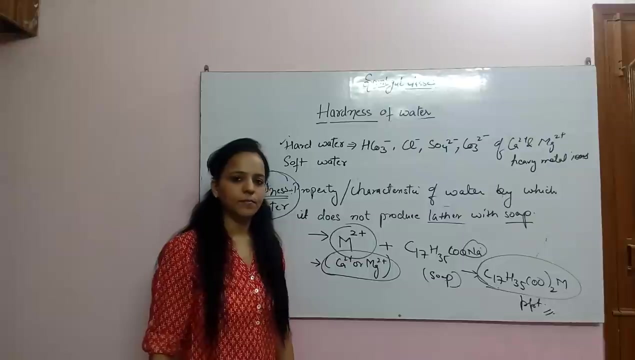 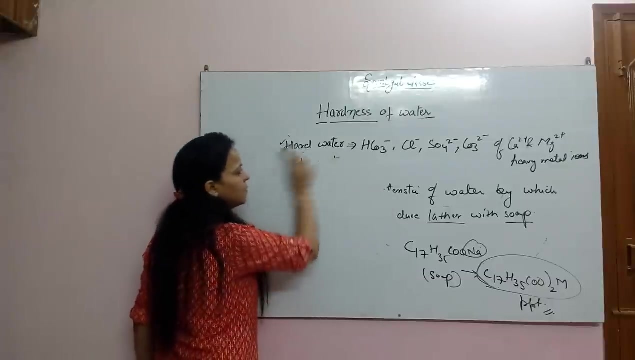 In water, And this property Of water, Due to which it does not produce Leather with soap, is known as Hardness of water. This property is known as Hardness of water. Hardness of water. Is it clear Next? Now we will see That Our water Is hard. 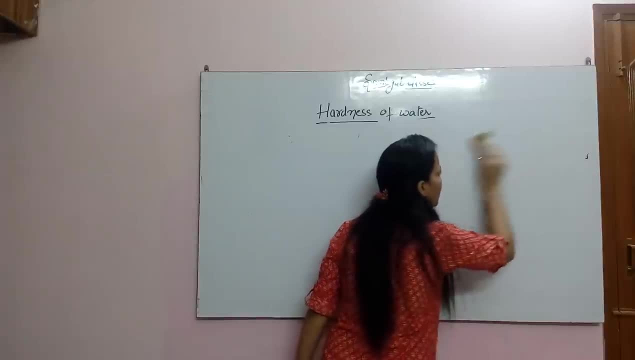 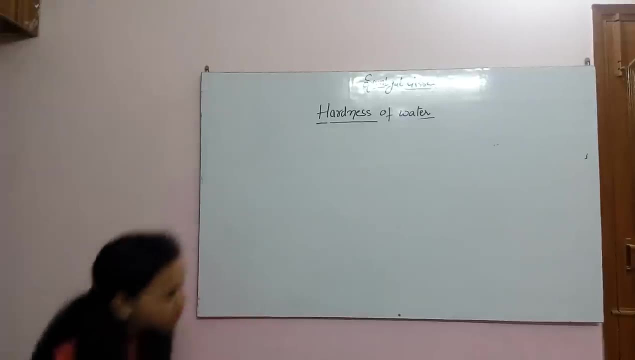 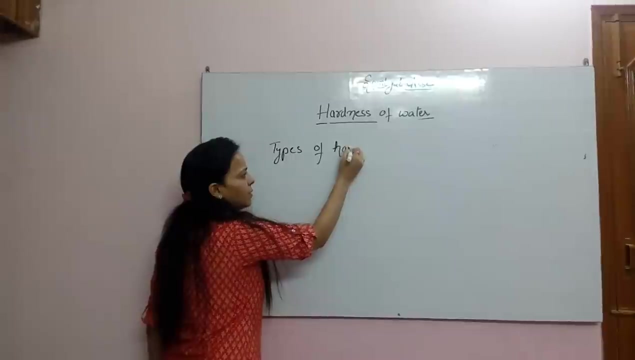 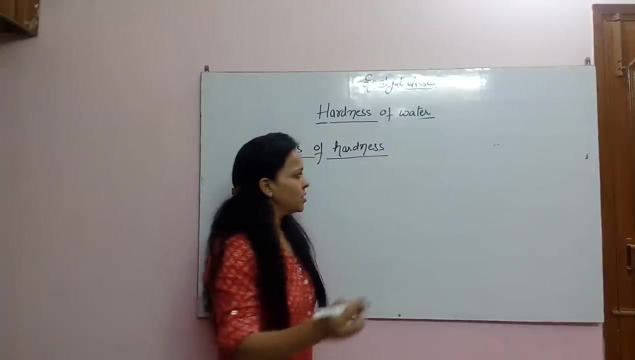 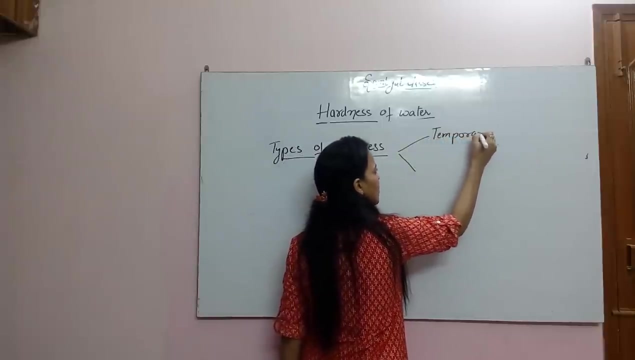 And your property is Hardness of water. Next we will see types of hardness. Next topic is Types of hardness. Types of hardness. Next is Types of Hardness. Types of hardness means There are two types of hardness. First is Temporary hardness- Temporary hardness- Temporary hardness. And the second is 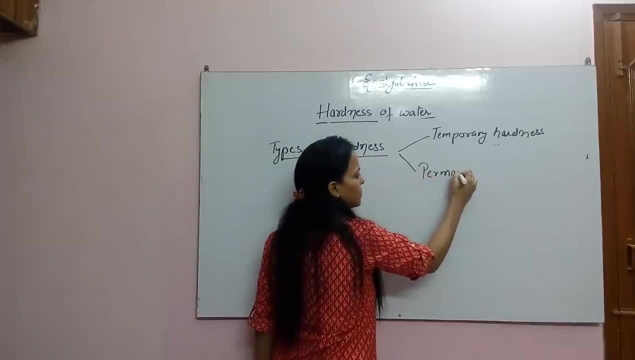 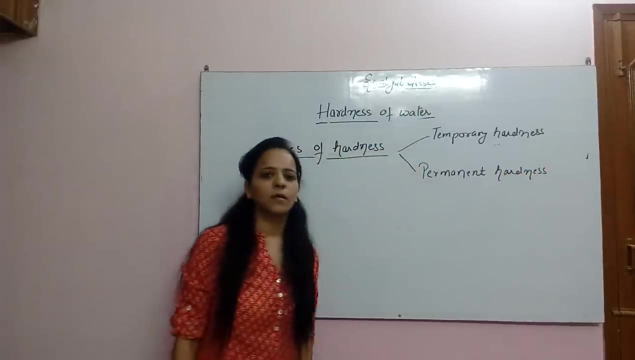 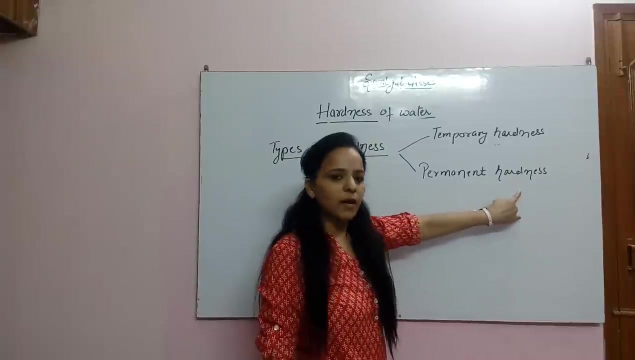 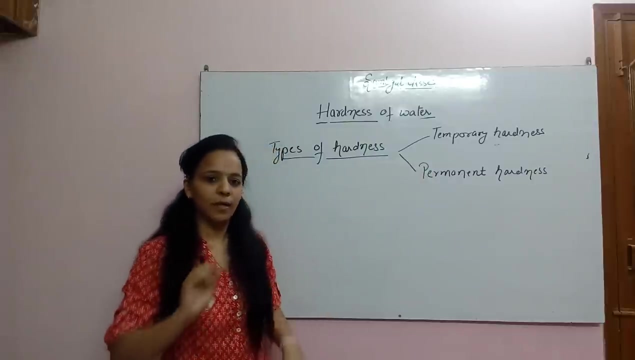 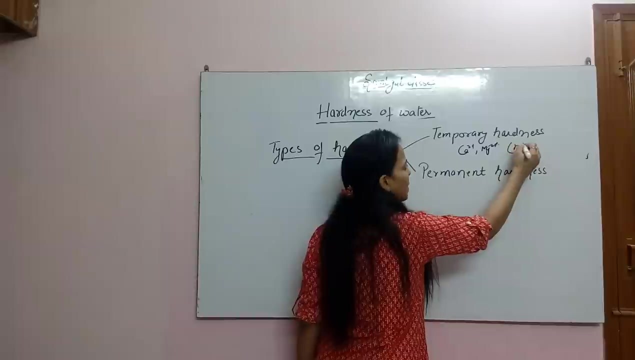 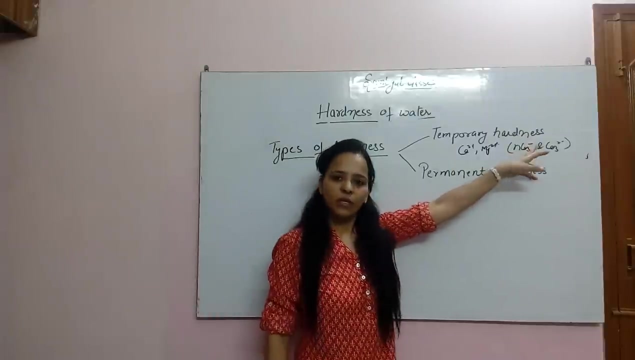 Permanent hardness, Permanent hardness, Hardness- two types of hardness: temporary hardness and permanent hardness. now see, temporary hardness will be due to calcium and magnesium metal ions present in water: bicarbonate ion and carbonate ion. ok, temporary hardness of water is due to the presence of. 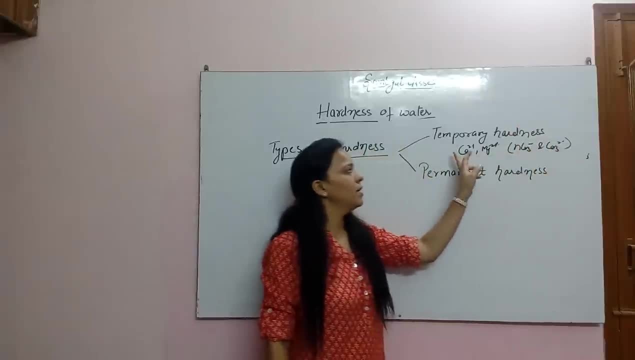 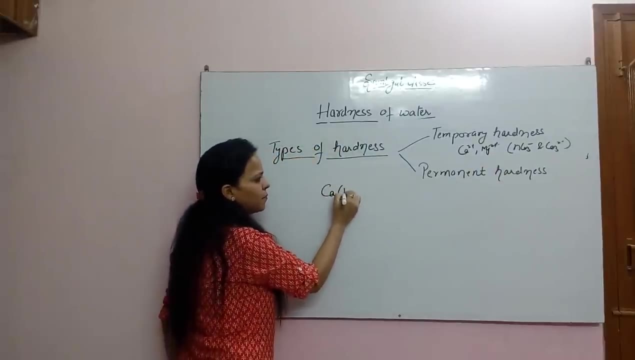 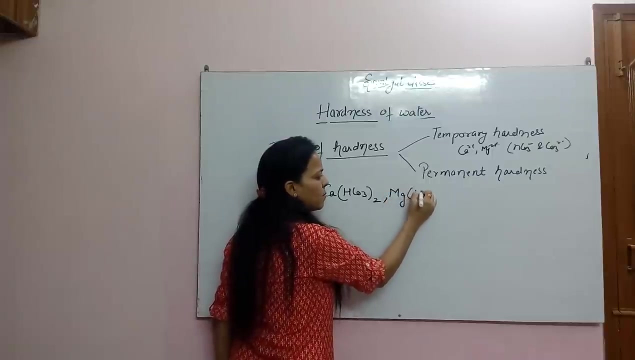 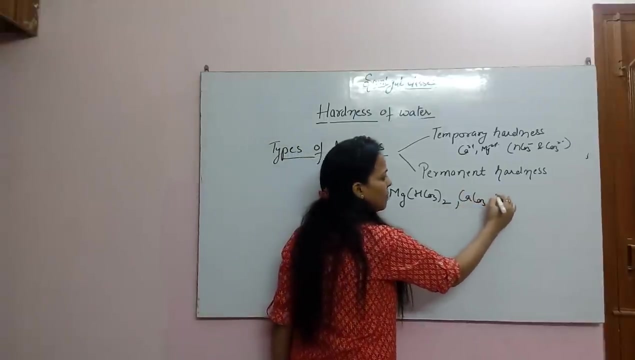 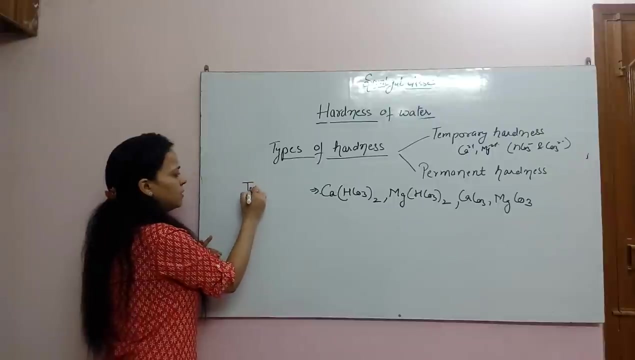 bicarbonate and carbonate ions of calcium and magnesium, for example. we see, now we have calcium bicarbonate- ok, magnesium bicarbonate- ok. now we have calcium bicarbonate- ok, clear calcium carbonate, magnesium carbonate. then all these salts are temporary hardness. 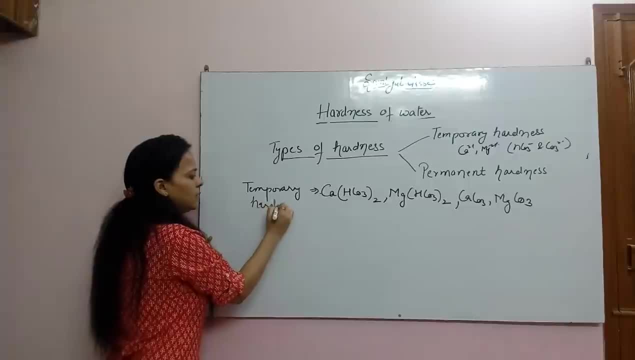 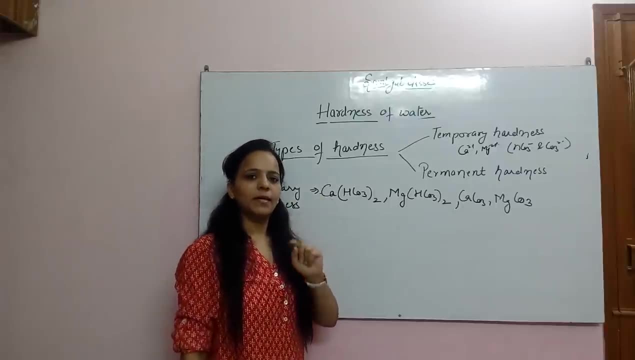 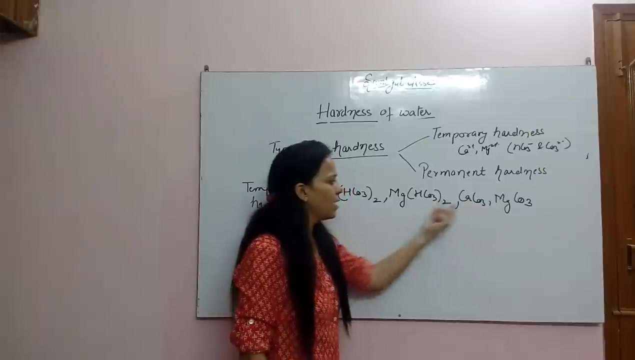 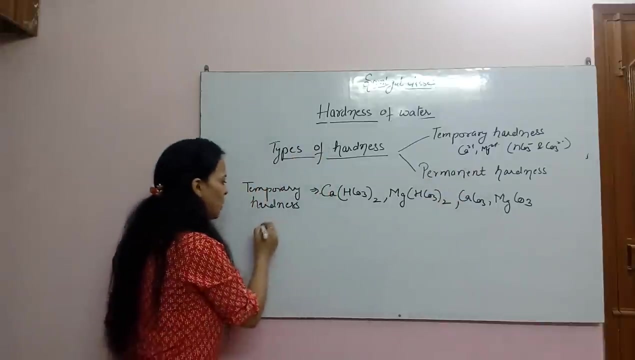 salts. these are temporary hardness salts clear which ions are responsible for temporary hardness: bicarbonate and carbonate ions, whose bicarbonate and carbonate ions of calcium, calcium and magnesium ions clear. similarly, your permanent hardness. permanent hardness is permanent hardness of water that is due to presence of, like our bicarbonate and carbonate. 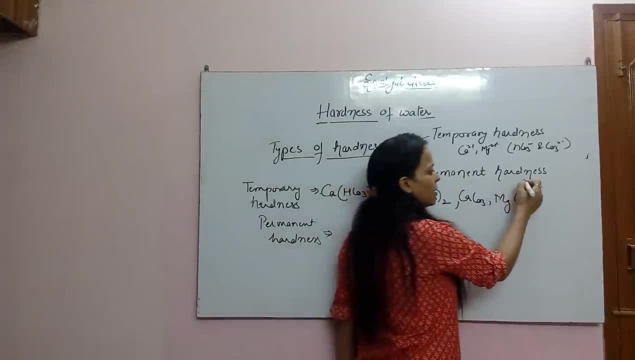 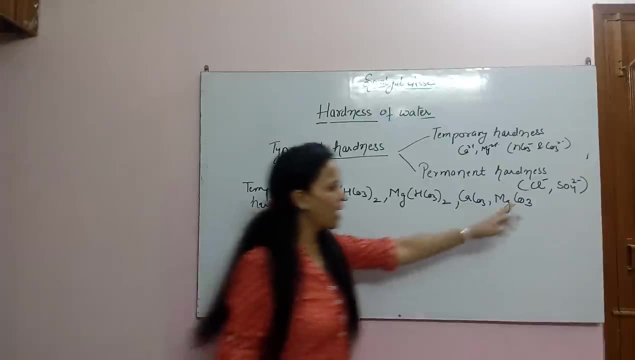 ions because of your temporary hardness. similarly, permanent hardness is due to the presence of chloride and sulphate ions. which ones? chloride and sulphate ions? ok. so bicarbonate and carbonate ions? Ok. So bicarbonate and chloride and sulphate ions? which ones? obviously, calcium and magnesium. 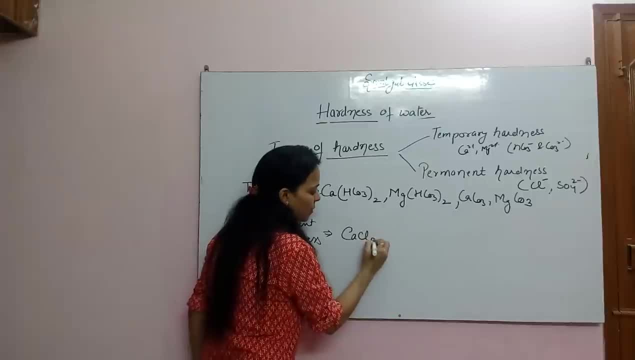 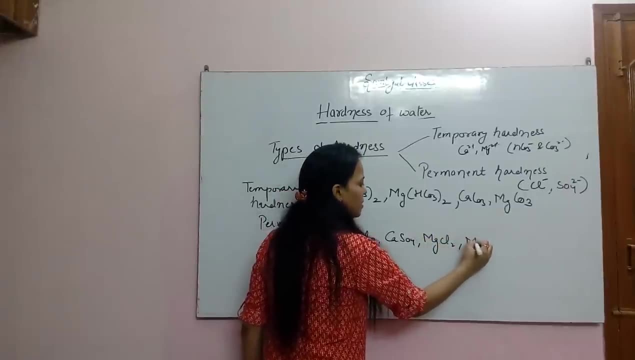 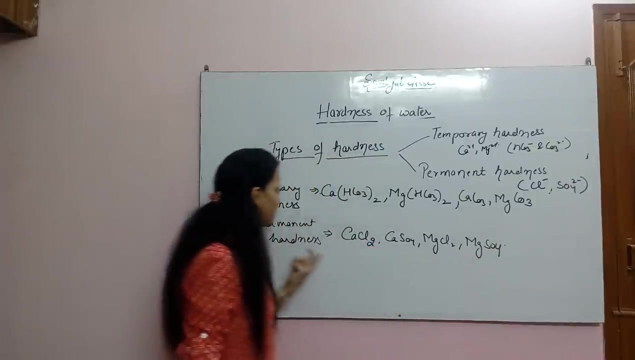 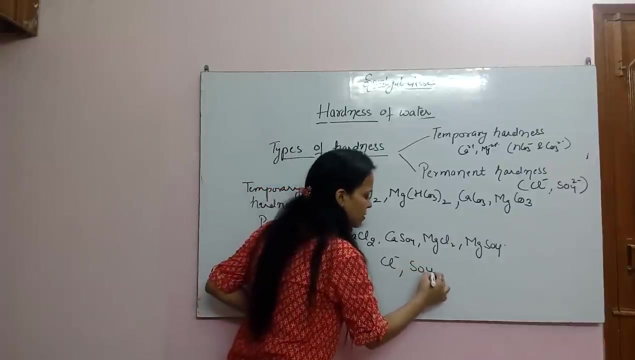 ions. now what we will do? now suppose we have calcium chloride, calcium sulphate, magnesium chloride and magnesium sulphate clear. so these salts, which hardness examples are there? permanent hardness. so permanent hardness is due to the presence of chloride and sulphate. 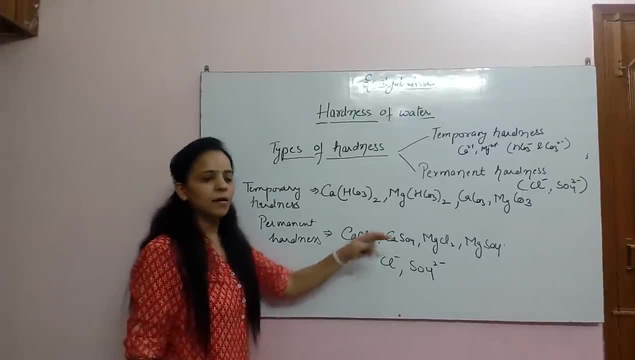 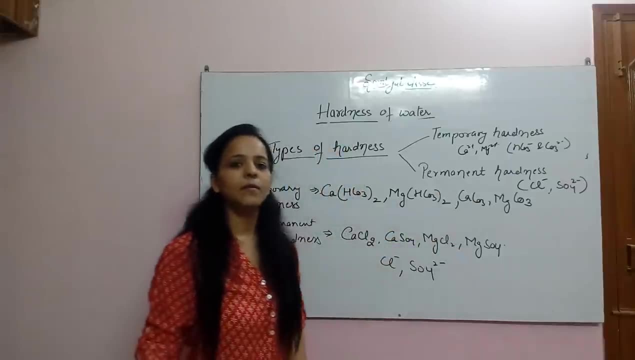 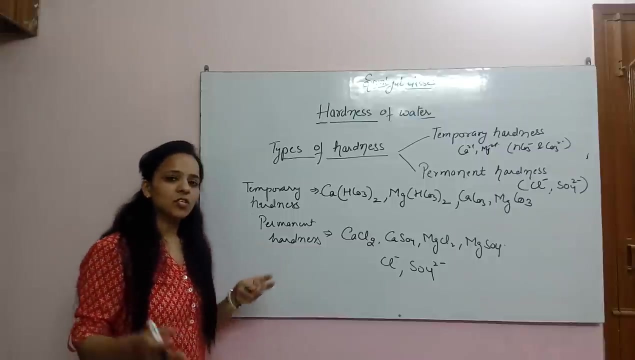 ions. ok, So these are the elements of calcium and magnesium ions, And temporary hardness is due to the presence of bicarbonate and carbonate ions of calcium and magnesium. Clear Temporary hardness. temporary means those which are for a short time. permanent means 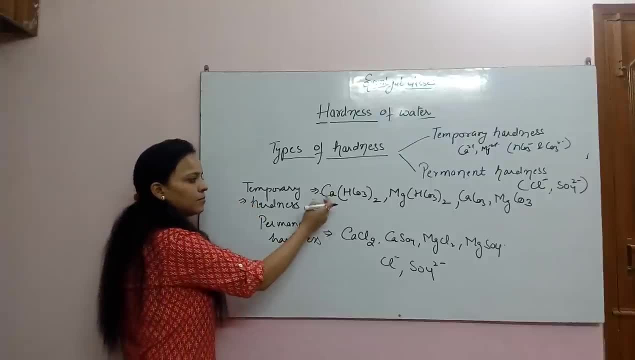 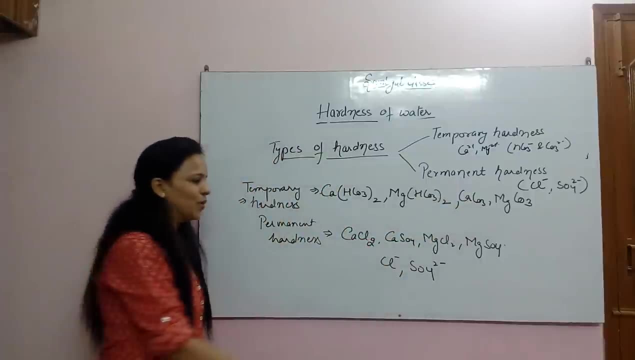 those which are not easily removed, which have been there for a long time. to remove them we have to see many methods. Temporary hardness- Do you understand vajasya aapki ki aapki hai. temporary hardness, chloride aur sulphate- times ki vajasya aapki. 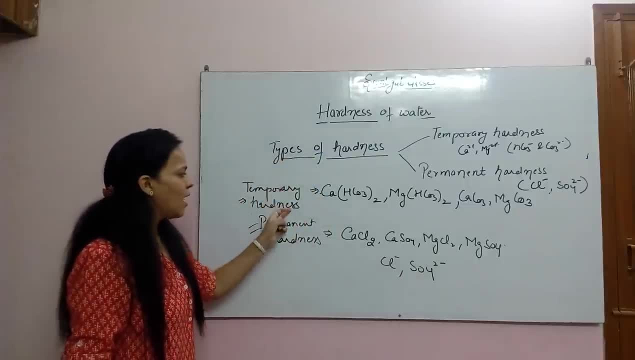 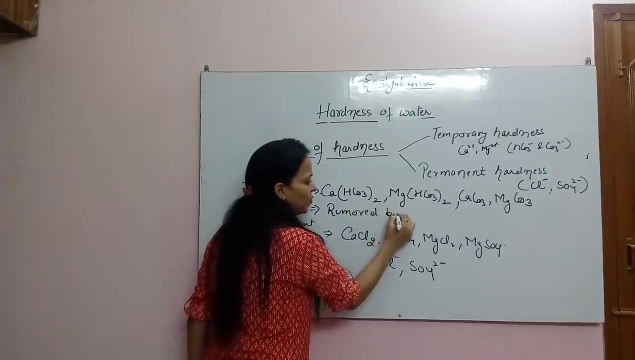 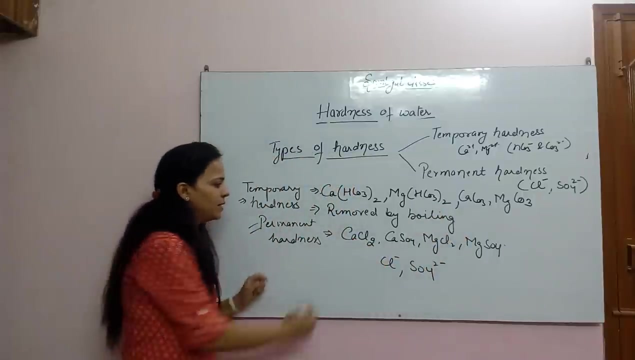 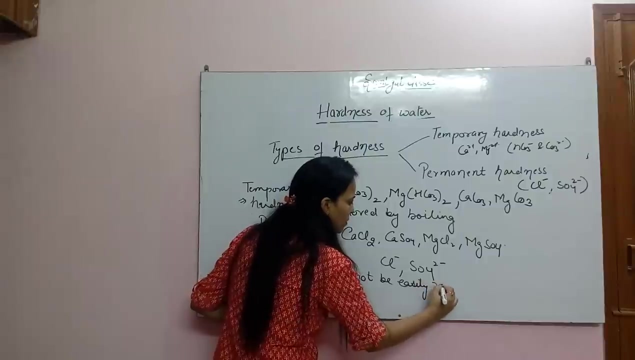 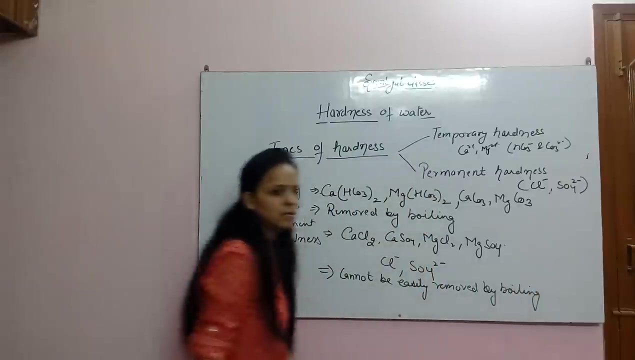 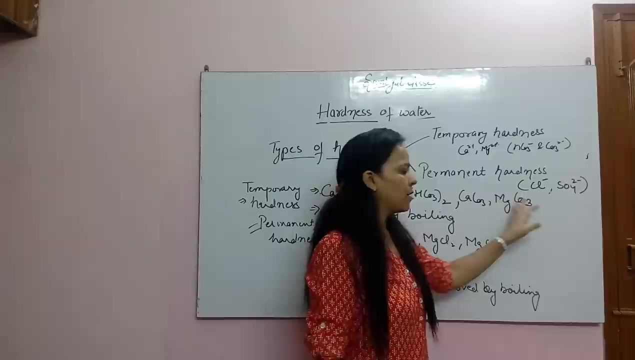 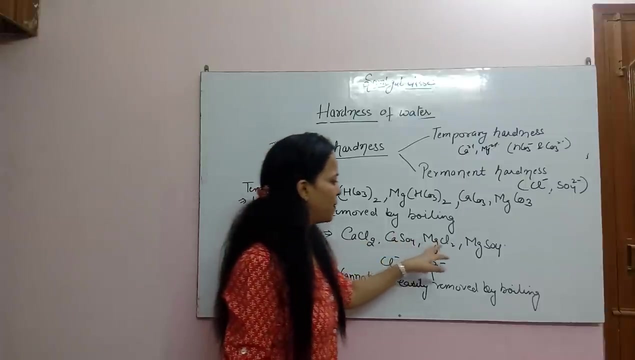 ki aapki hai permanent hardness, now temporary hardness, that can be removed by boiling. it can be removed by boiling clear, but permanent hardness cannot be easily. cannot be easily removed by boiling. yeah, calcium bicarbonate, magnesium bicarbonate, calcium carbon, magnesium bicarbonate- these are all examples of temporary hardness. and calcium chloride, calcium sulphate.